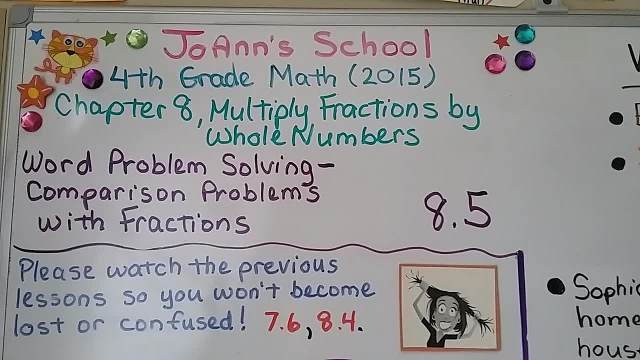 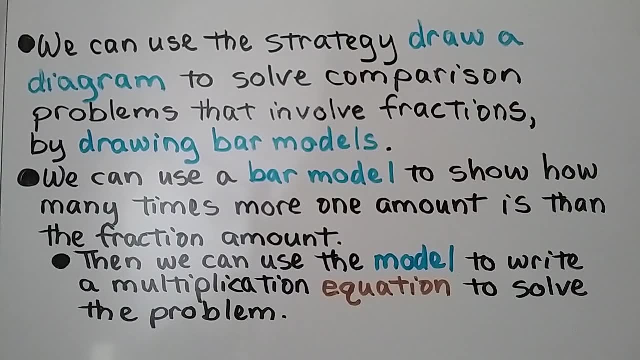 Lesson 8.5 Word Problem: Solving Comparison Problems with Fractions. We can use the strategy Draw a Diagram to solve comparison problems that involve fractions by drawing bar models. We can use a bar model to show how many times more one amount is than the fraction amount. Then we can use the model to write a multiplication equation. 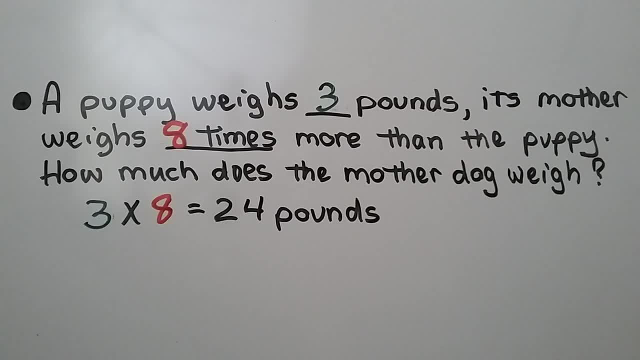 to solve the problem. A puppy weighs three pounds. Its mother weighs eight times more than the puppy. How much does the mother dog weigh? The puppy weighs three pounds. The mother weighs eight times more. We do three times eight, which is equal to twenty-four. 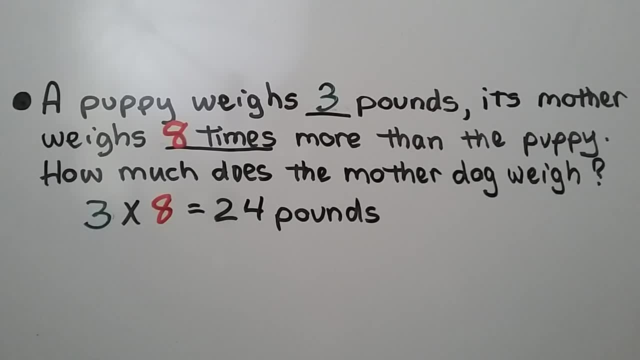 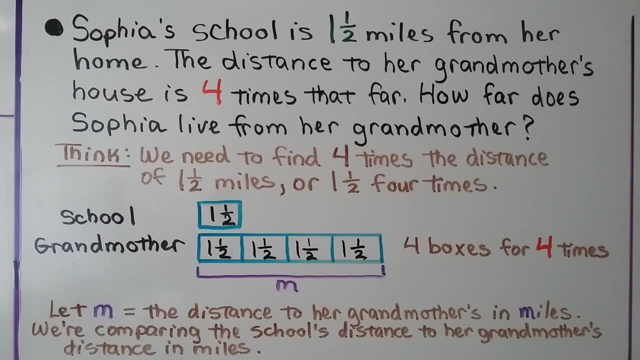 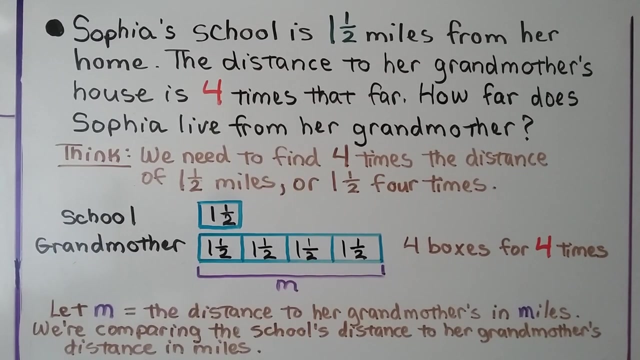 pounds. We know the mother dog weighs twenty-four pounds. Sophia's school is one and a half miles from her home. The distance to her grandmother s house is four times that far. How far does Sophia live from her grandmother? So we need to find four times the distance of one and a half miles, or one and a half. 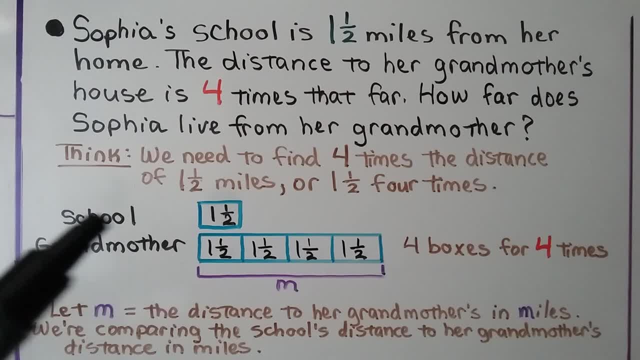 four times. We use a bar model and we show: the school is one box, one and a half, and the grandmother is four times that. so we have four boxes for four times. And do you see this, M? We're going to let M equal the distance to her grandmother's house in miles. Miles starts. 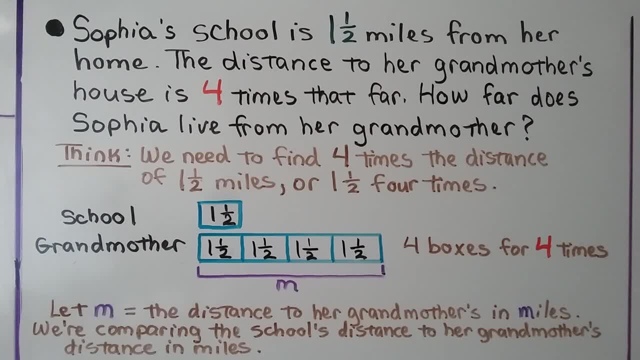 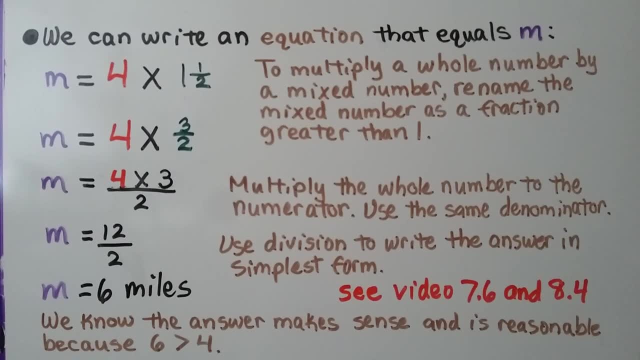 with M see We're comparing the school's distance to her grandmother's distance in miles. We can write an equation that equals M. for miles, M is equal to four times one and a half. And to multiply a whole number by a mixed number, we rename the mixed number as: 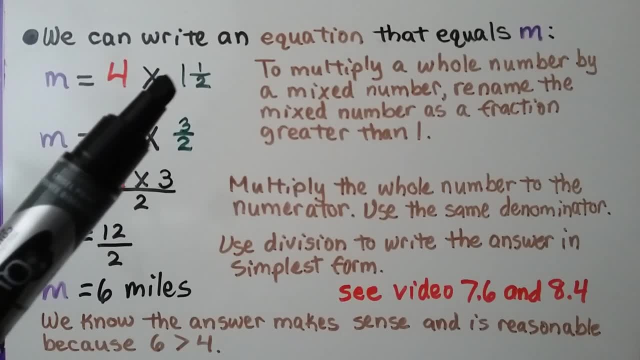 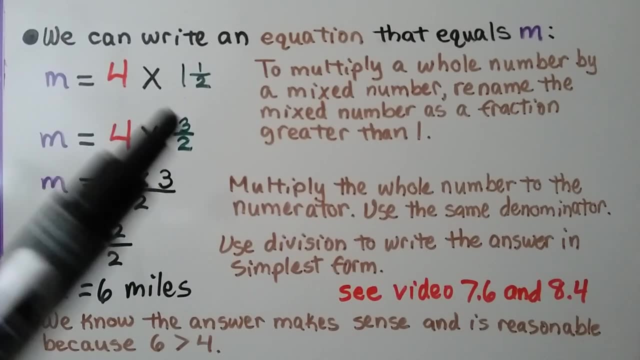 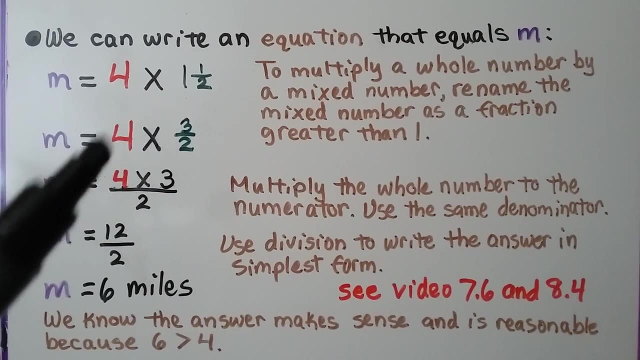 a fraction greater than one. We do one times the denominator two plus the numerator one. That's going to give us three halves. We learned how to do this in the last few videos. Now we multiply four times three halves. by multiplying the four to the numerator three, We write: 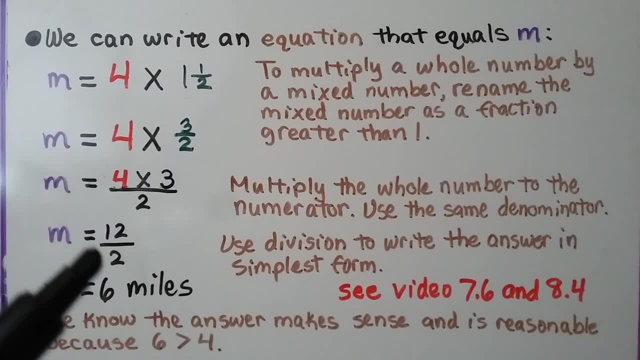 it over that denominator two, We get twelve halves, And then we use division to write the answer in simplest form: Twelve divided by three equals one. And then we do the same: 12 divided by 2 is equal to 6.. We know m is equal to 6 miles. 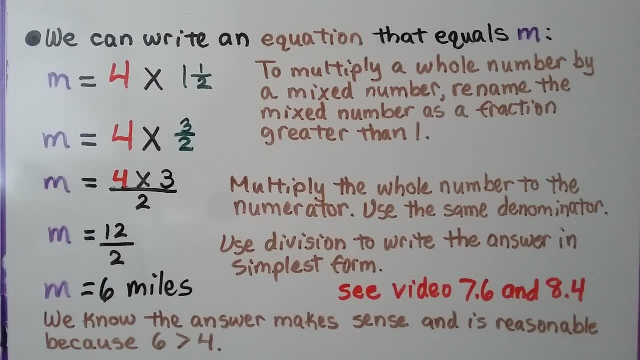 We know Sophia lives 6 miles from her grandmother. We also know the answer makes sense and is reasonable because this 6 is greater than this factor 4, the whole number. We also learned that when we multiply a number by a mixed number, the product will be greater. 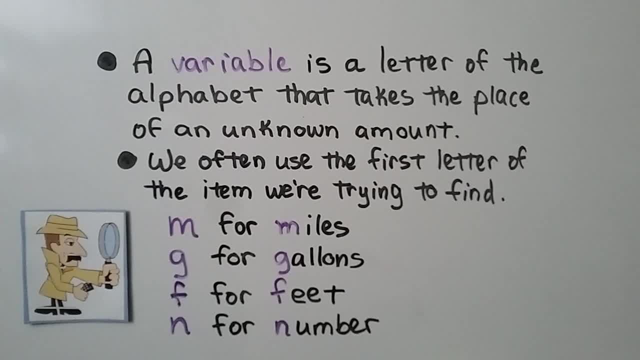 than the whole number. We've also learned before that a variable is a letter of the alphabet that takes the place of an unknown amount. We often use the first letter of the item we're trying to find. So we'll use an m for miles, or a g for gallons, or f for feet or an n for number. 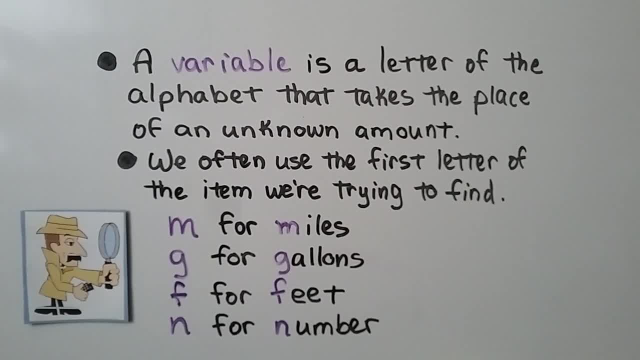 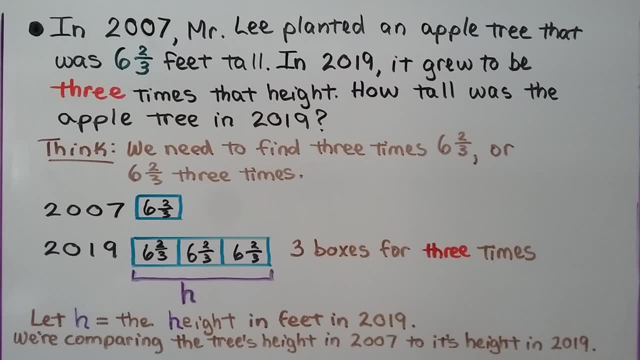 We might also see a p or a q or an r. We might also see an x. In 2007,, Mr Lee planted an apple tree That was 6 and 2 thirds feet tall. In 2019, it grew to be 3 times that height. 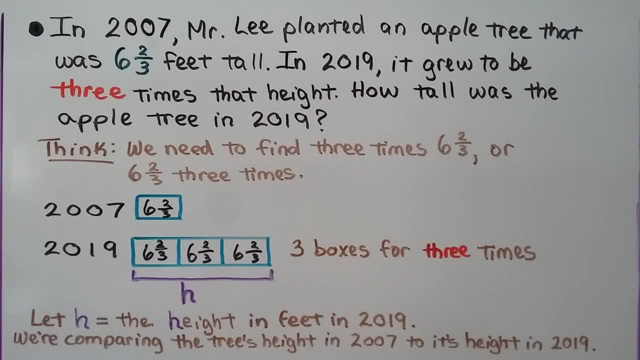 How tall was the apple tree in 2019?? So we think we need to find 3 times, 6 and 2 thirds, or 6 and 2 thirds 3 times. We use a bar model to show that it was 6 and 2 thirds feet in 2007 and we use 3 boxes in. 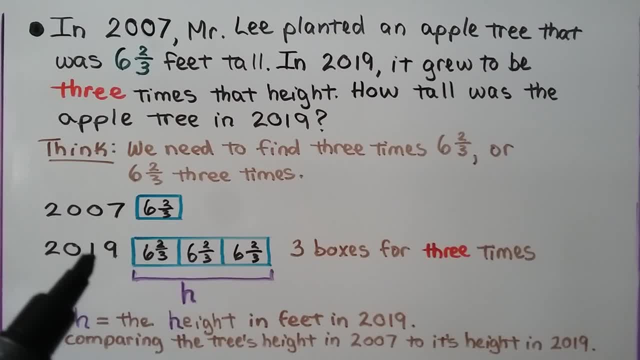 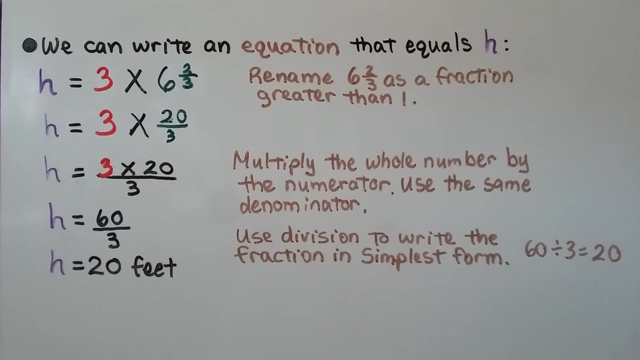 our bar model for 3 times for 2019.. And these 3 boxes are going to equal the height in feet in 2019.. We're comparing the tree's height in 2007 to its height in 2019.. We can write an equation that equals h- the height in feet. 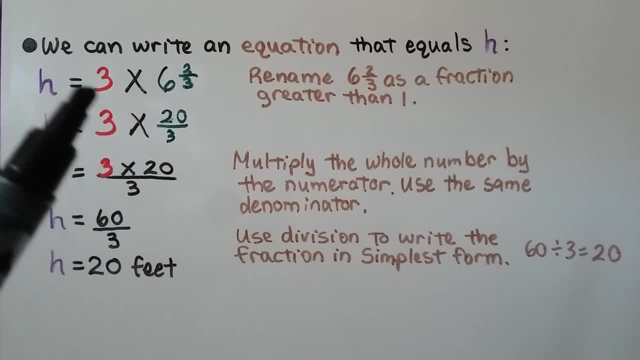 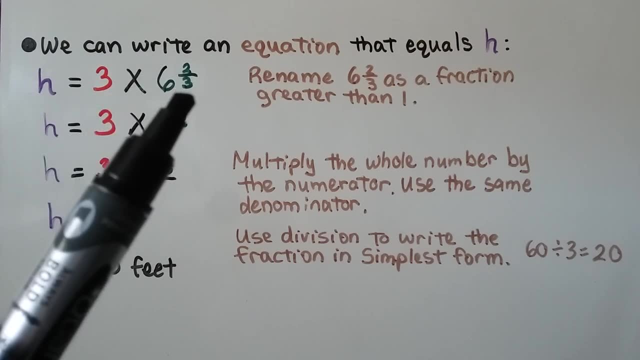 H is equal to 3 times 6 and 2 thirds. We can write an equation that equals h, the height in feet. Can we multiply these? We rename the 6 and 2 thirds as a fraction greater than 1.. We do 6 times the denominator 3, that's 18.. 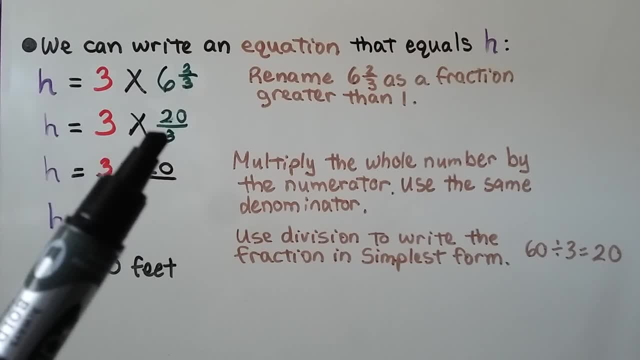 We add the 2 numerator and we get 20.. We write it over that 3 denominator, we have 20 thirds, And 3 times 20 thirds is 3 times 20.. This, 3 times the numerator over that 3 denominator, we get 60 thirds. 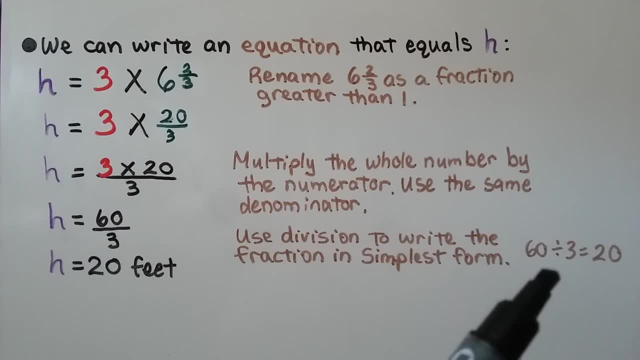 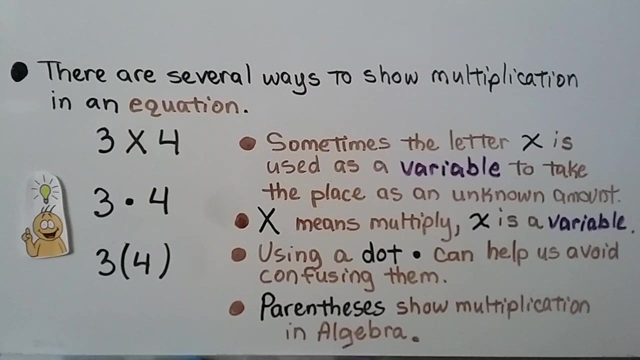 We use division to write the fraction in simplest form. We think 60 divided by 3. three is equal to 20, it's 20 feet tall in 2019.. And there are several ways to show multiplication in an equation. We've been using this big X for three times four. 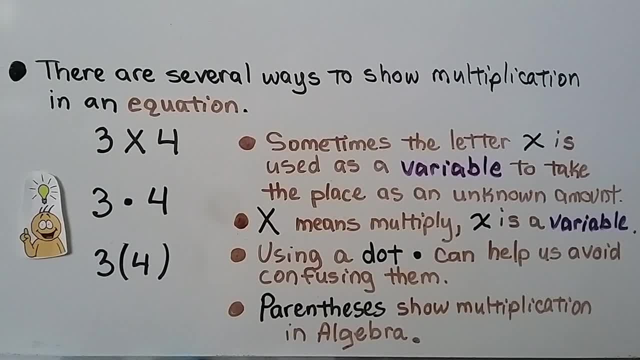 Well, sometimes a letter X is used as a variable to take the place as an unknown amount. This big X means multiply. If you see the X written like this, it's a variable, It's taking the place of an unknown amount And using a dot in between the two numbers. 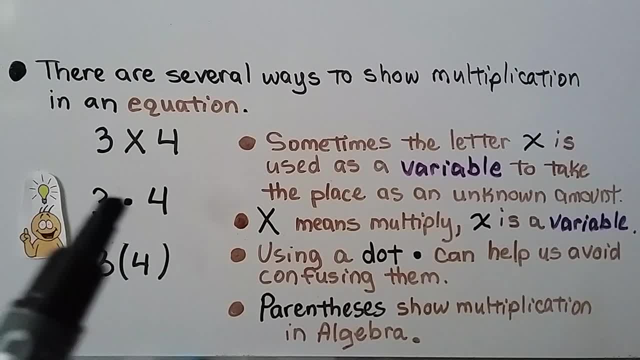 can help us avoid confusing them. Some people use a dot. My granddaughter does. Parentheses also show multiplication. You're gonna use this in algebra. The number will be right up next to the parentheses. You won't see an operation sign in between them. 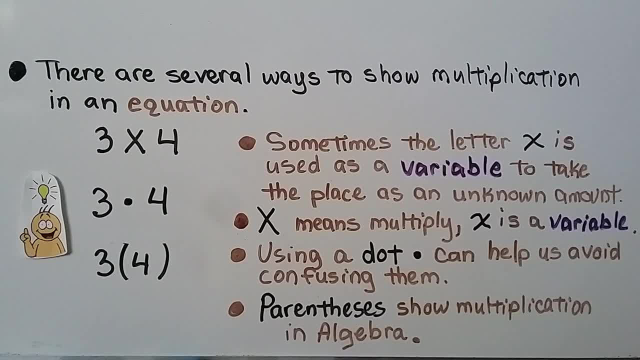 That means we're multiplying three times four. So variables are usually written in what's called italics. It almost looks a little bit script or slanted. So you know if it's a really big X like this it means multiply. The average weight of a 12 week old kitten is three pounds. 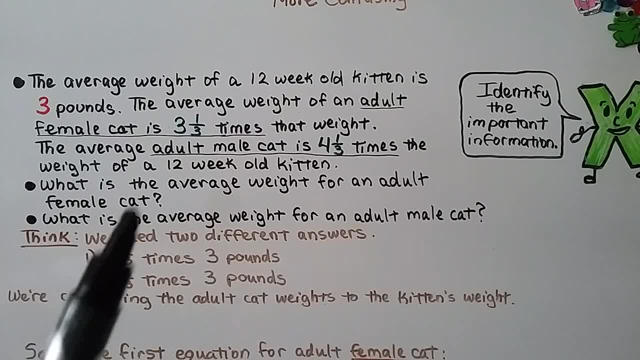 The average weight of an adult female cat is three and one third times that weight. The average adult female cat is three and one third times that weight. The average adult female cat is three and one third times that weight. adult male cat is four and one-third times the weight of a 12 week old kitten. 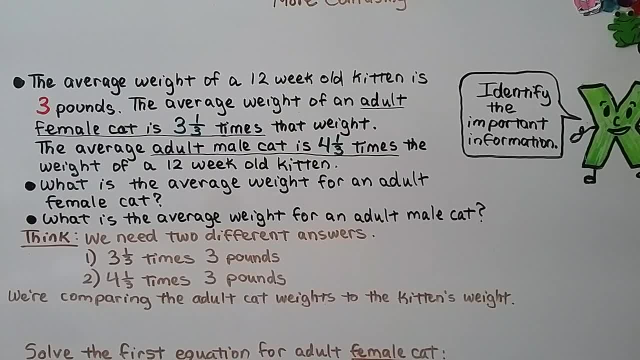 What is the average weight for an adult female cat? What is the average weight for an adult male cat? So we need two different answers: The average weight for the adult female and the average weight for the adult adult male. We need to identify the important information. It's not important that the kitten is 12. 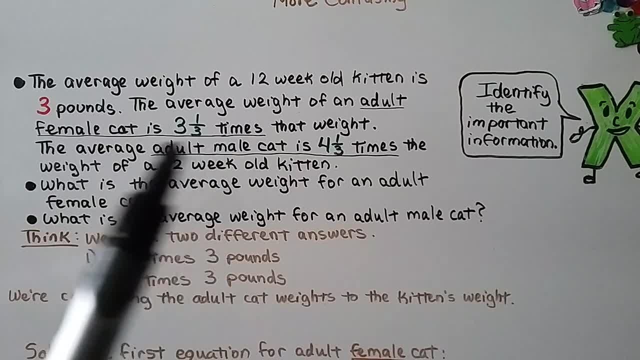 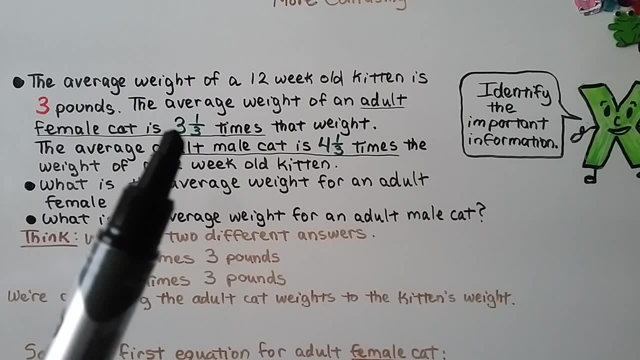 weeks old, So that number 12 is not going to help us, But it is important that the kitten is 3 pounds. It's also important that the adult female cat is three and one-third times this 3 pounds, And it's important that the average 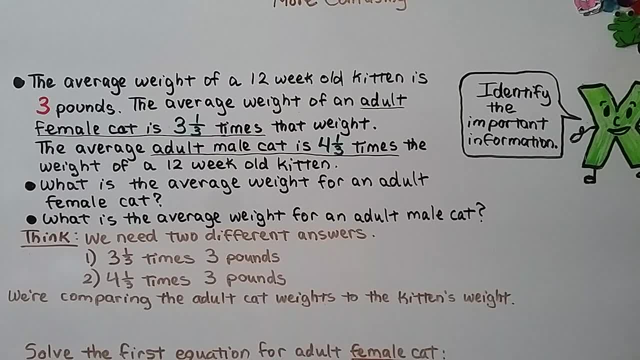 adult male cat is four and one-third times that, 3 pounds. So we're going to have two different answers: Three and one-third times 3 pounds and four and one-third times 3 pounds. That's two different equations. We're comparing the adult cat's weights to the kitten's weight. We solved the. 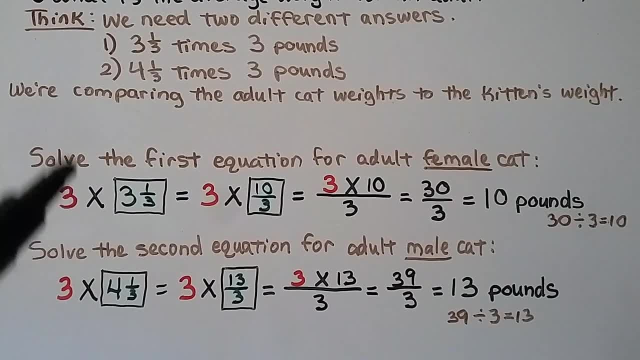 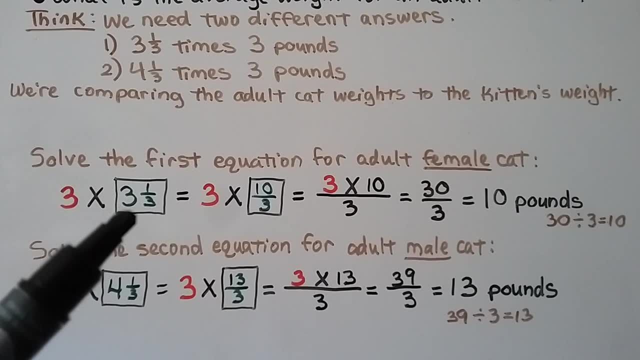 first equation for the adult female cat. We're going to do three times three and one-third. We're going to write this mixed number as a fraction greater than one. We do three times three plus one. That gives us a ten-thirds. We multiply. 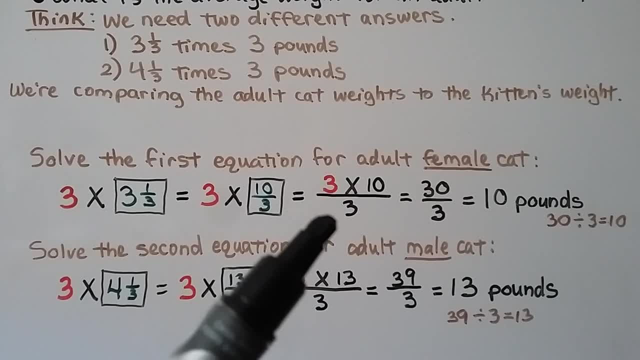 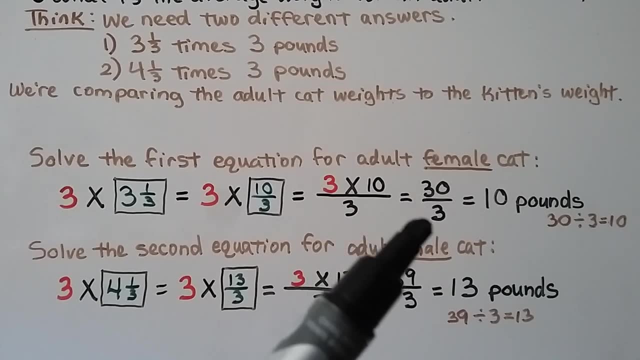 the whole number to the numerator, We have three times ten over that three denominator, That's thirty-thirds. We use division to simplify this. to put it in simplest form, That's thirty divided by three is equal to ten. So we know the average adult female cat is ten pounds. Now we do it for the adult male cat. We. 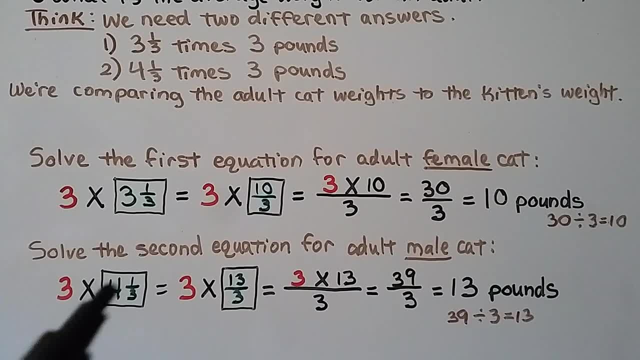 have three times four and one-third. We put this mixed number into a fraction greater than one. We do the four times three denominator, which is 12.. We add the numerator, that's 13,. we use the same denominator. we have 13 thirds. 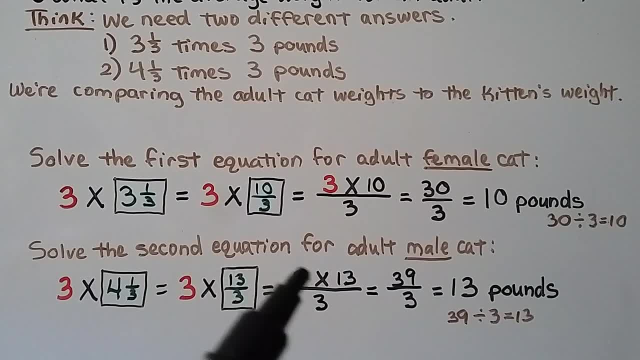 We multiply the whole number to the numerator three times 13,. that's equal to 39.. We use the same denominator, we have 39 thirds. We write this in simplest form by doing division: 39 divided by three is equal to 13.. So we know the average adult male cat is 13 pounds. A bird's wingspan is the total length from one outstretched wing tip to the other, all the way across its body. that's its wingspan. We have a table here showing birds of prey wingspans. 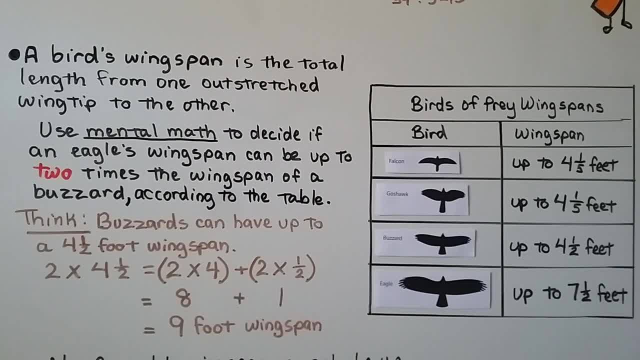 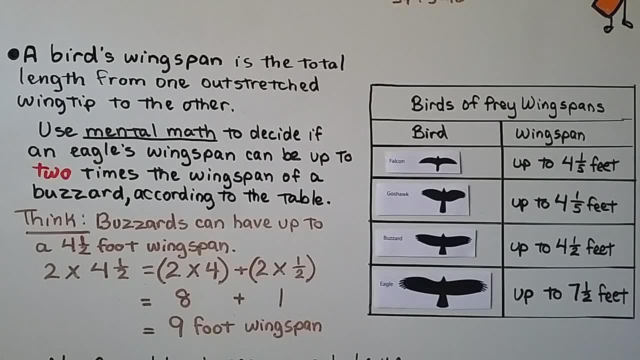 We have a falcon, a goshawk, a buzzard and an eagle, And it's showing that a falcon's wingspan can be up to four and one fifth feet And a goshawk can have a wingspan up to four and one fifth feet, just like the falcon. 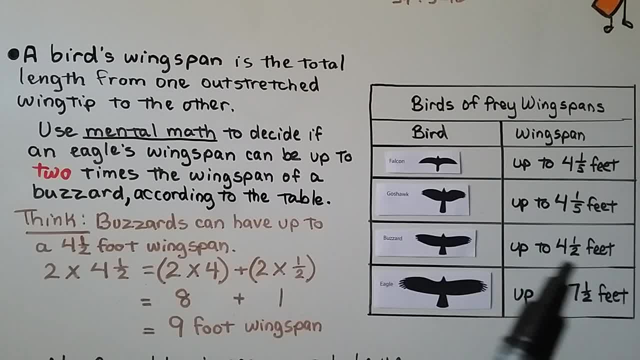 And the buzzard is up to four and one half feet, so it could be less. that's just how far it can go up to usually. And then the eagle goes up to seven and a half feet. It's telling us to use mental math. 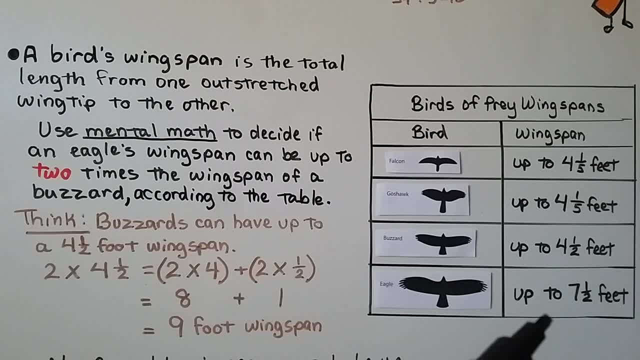 to decide if an eagle's wingspan can be up to two times the wingspan of a buzzard, according to this table table. So we need to do 2 times 4 and a half. 2 times 4 is 8.. Then we have to do 2 times. 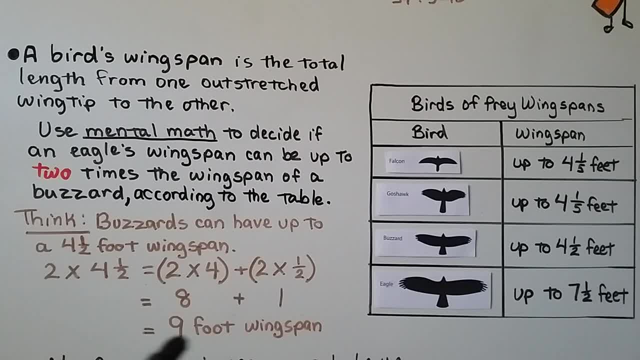 a half, That's one whole. We have two halves. That's a 9 foot wingspan, And we can use mental math doing this. We multiply the 2 to the 4. We get an 8. Then we multiply the 2 to the. 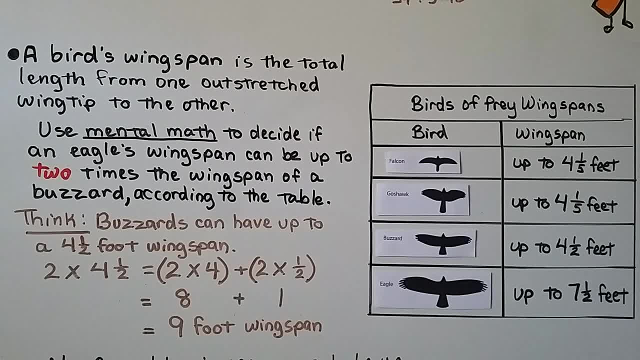 half and we get one whole. So a buzzard's wingspan times 2 would be up to 9 feet. Oh, that's too big, That's too great. This is only 7 and a half feet, So the answer is no. 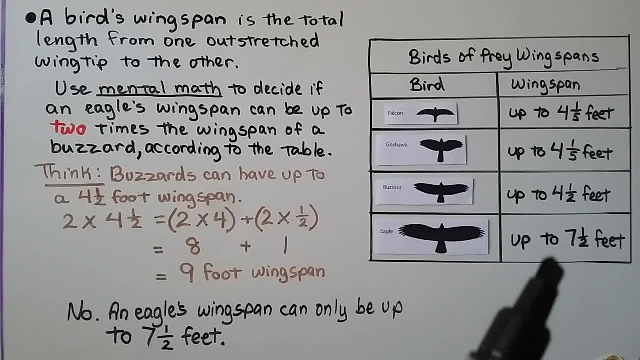 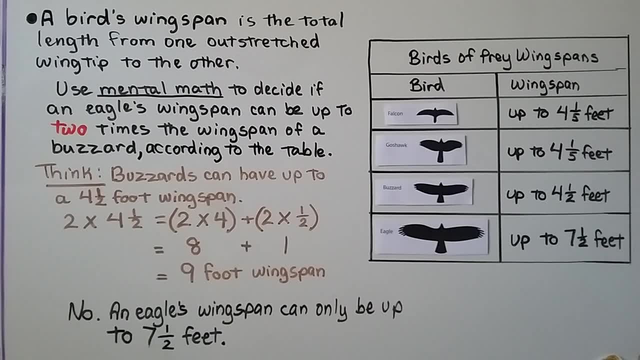 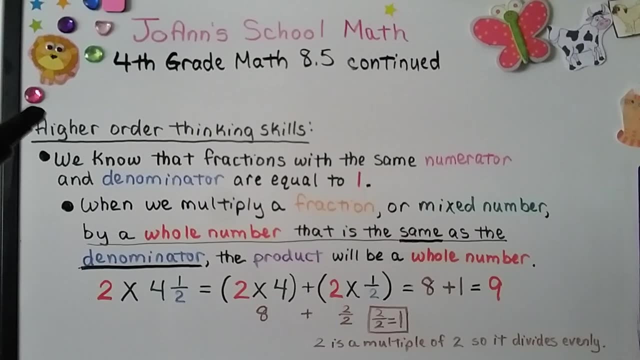 An eagle's wingspan can only be up to 7 and a half feet according to this chart. It can't be 2 times that of a buzzard. Now let's do some higher order thinking skills. We know that fractions with the same numerator and 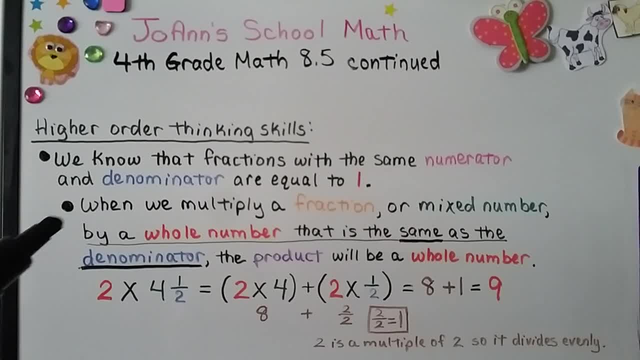 denominator are equal to 1, one whole. Well, when we multiply a fraction or mixed number by a whole number- that is the same as the denominator- the product will be a whole number. When we multiply a fraction or mixed number by a whole number, that's the same as the denominator. 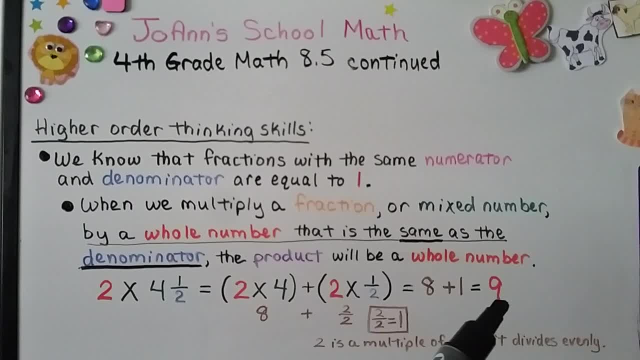 see we have a 2 and the denominator is a 2? Then we know the product's going to be a whole number. Let's see how this worked. We would do 2 times 4, that's 8.. Then we would do 2 times this half. Well, that's 2 halves. We have an 8 plus 1, that's equal to 9.. And this numerator 2 is a multiple of this denominator 2, so it divides evenly. We have a whole number. Let's try that again. 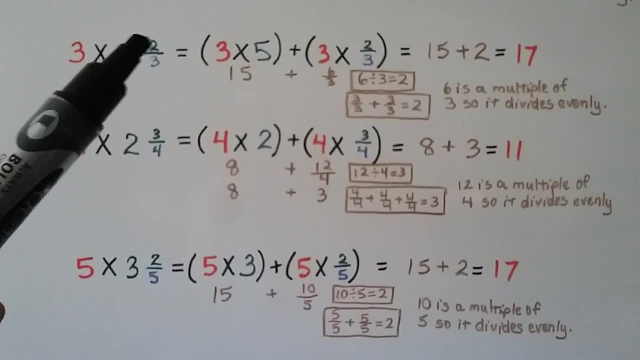 Now we have 3 times 5 and 2 times 2.. That's a whole number. Let's try that again. 2 thirds. look, we have a 3 here and a 3 here. We know the answer is going to be a whole. 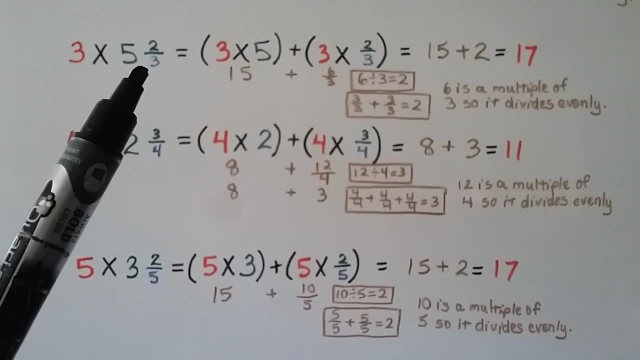 number, because that's a 3 and in the mixed number the denominator is a 3.. We start by doing the 3 times 5, that's 15, then we do 3 times the 2 thirds. We multiply the 3 to. 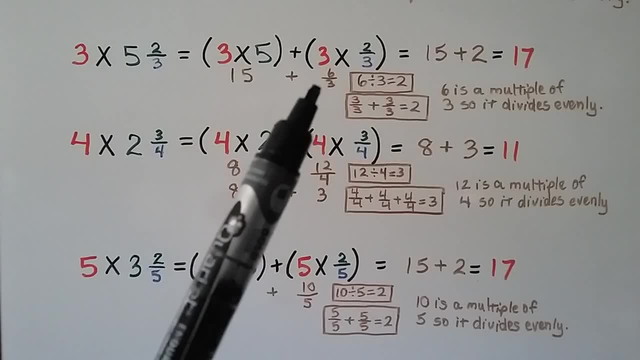 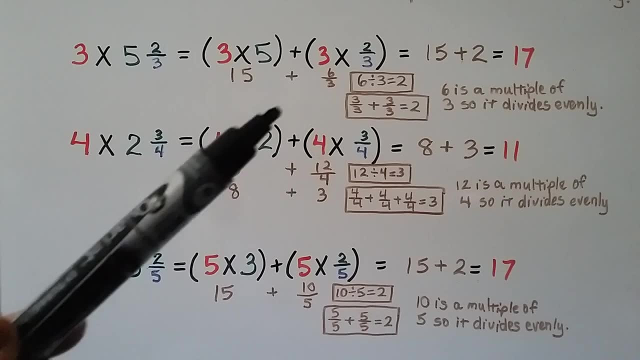 the numerator 2, that's 6 thirds, And 6 divided by 3 is 2.. It's like a 3 thirds plus 3 thirds. that's equal to 2.. And this numerator 6 is a multiple of that denominator 3, so we know. 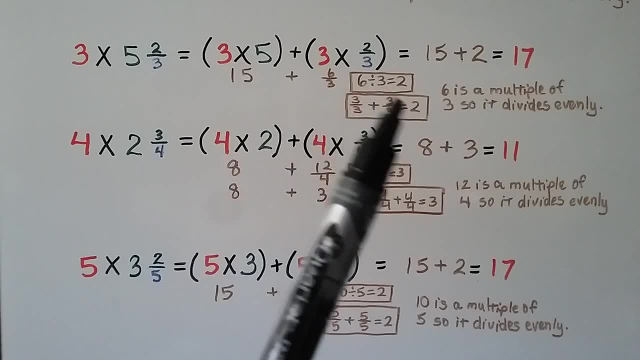 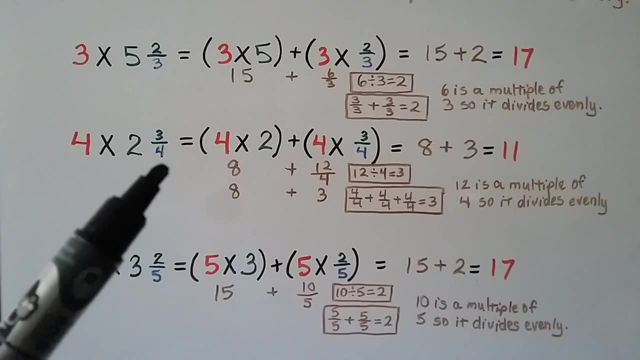 it divides evenly. Our answer is 15 plus 2, it's 17.. We have a whole number. Now, look, we have a 4 here and we have a denominator 4 here. We have 4 times 2 and 3 fourths, And 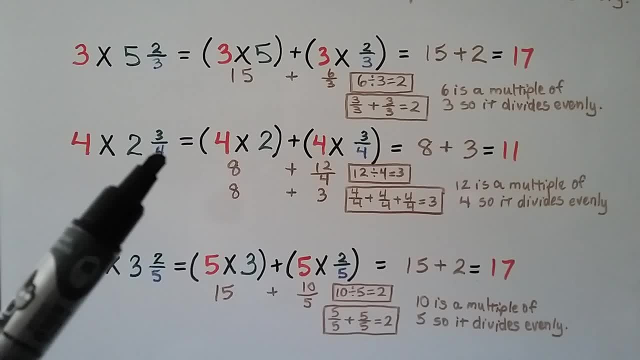 because that's a 4 in the whole number and that's a 4 in the denominator. we know our answer is going to be a whole number. The product is the denominator. We do the 4 times 2 first. that's going to give us an 8. Then we do 4 times 3, fourths. 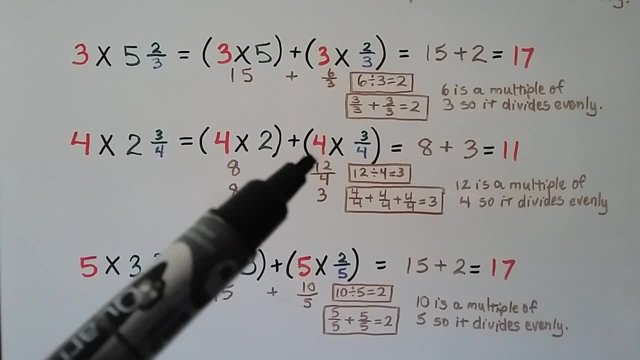 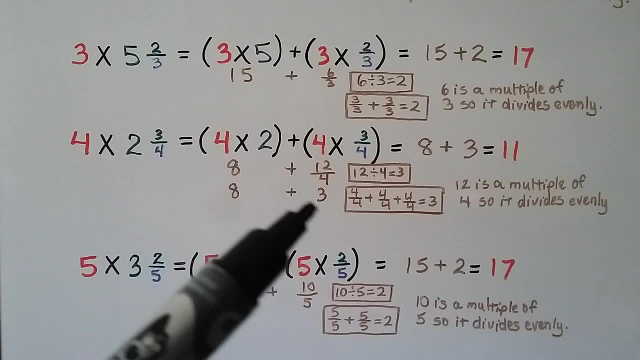 We multiply the 4 to the 3 numerator, we get 12 fourths. We divide. to put this in simplest form: 12 divided by 4 is a 3. So we're adding 8 plus 3 and that's 11. We have a whole number. 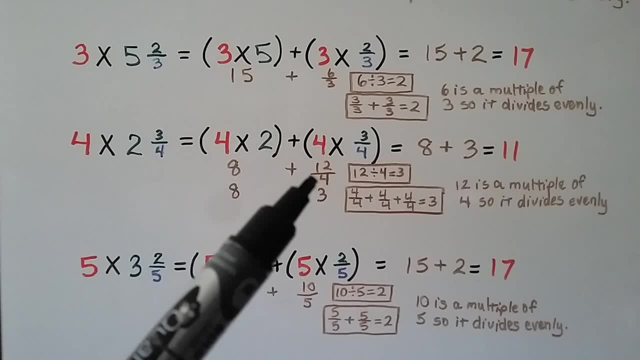 This 12 numerator is a multiple of this 4 denominator, so we know it divides evenly. Try it again. We have a 5 here and a 5 in the denominator of the mixed number. We know this is going to equal a whole number. We do the 5 times 3, which is 15.. Then we do: 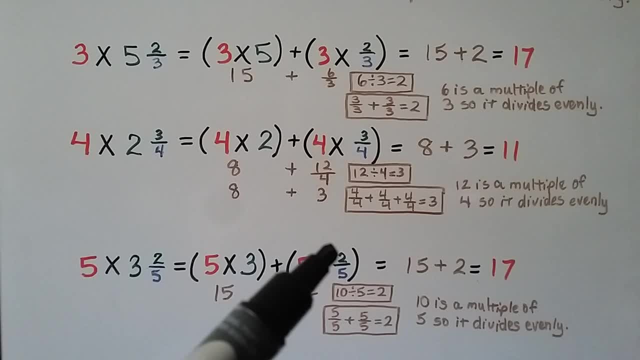 the 5 times 2 fifths. We multiply the 5 to the 2 numerator and get a 10.. That's 10 fifths, And we divide this. to put it in simplest form: 10 divided by 5.. That's a 2. We have 15 plus. 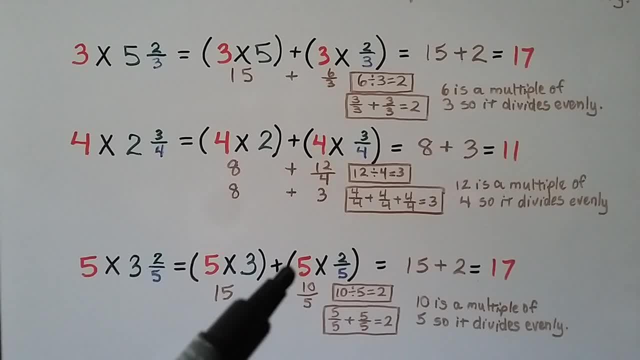 2,, that's a 17. This 10 numerator is a multiple of that 5 denominator and it divides evenly. So when this whole number is the same as the denominator of the fraction or mixed number, we know our answer is going to be a whole number. 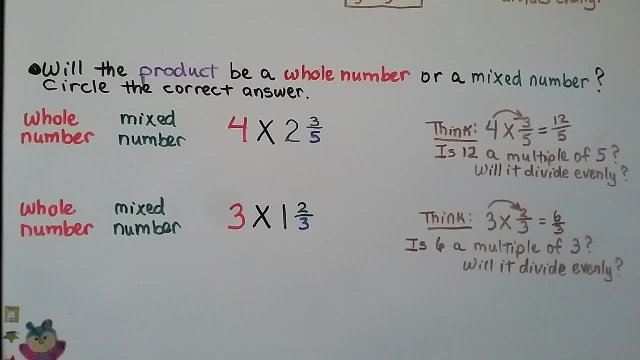 So will the product be a whole number or a mixed number? We need to circle the correct answer: Whole number or mixed number. Here we've got 4 times 2 and 3 fifths. Now look at this 4 and look at the denominator. 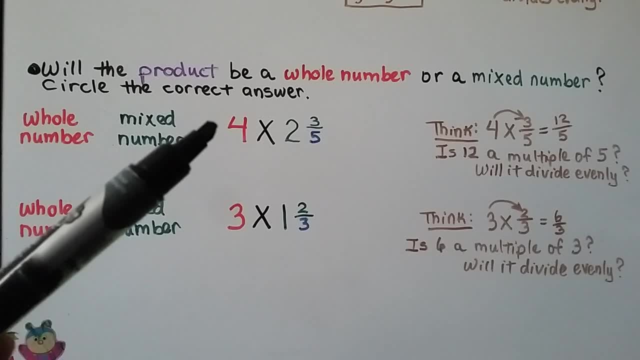 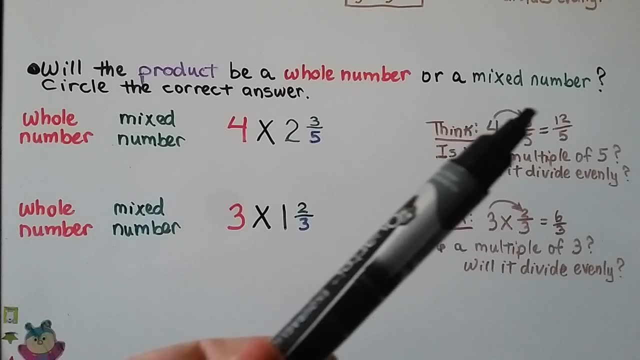 in the mixed number. We think when we get to the part where we're multiplying the 4 times the 3 fifths, we're going to multiply the 4 to the numerator of 3 and get a 12.. That's going to give us 12 fifths. And is 12 a multiple of 5? Will it divide evenly? 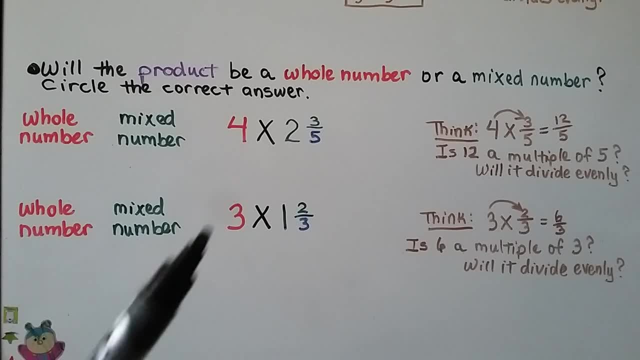 No, it won't. So we're not going to have a whole number, We're going to have a whole number. Now, we're going to have a whole number. We're going to have a whole number. We're going to have number. this 4 is not the same as the denominator here, so we're going to have. 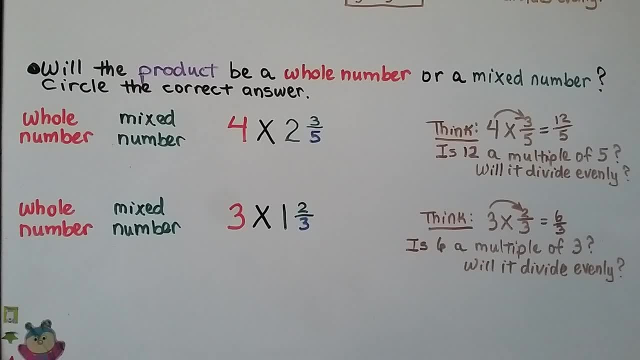 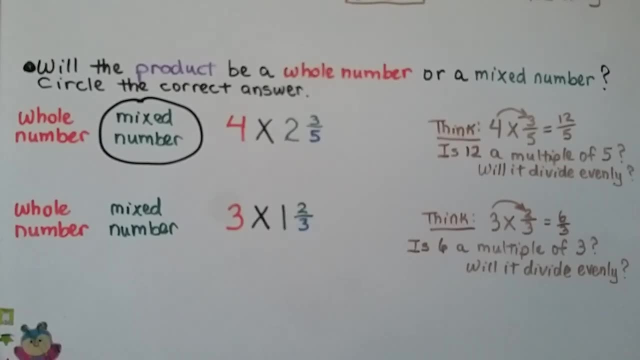 a mixed number for our product. now look at this one. is the product going to be a whole number or mixed number? we have 3 times 1 and 2 thirds. we see we have a 3 here and a 3 in the denominator. and we think, when we get to the part where 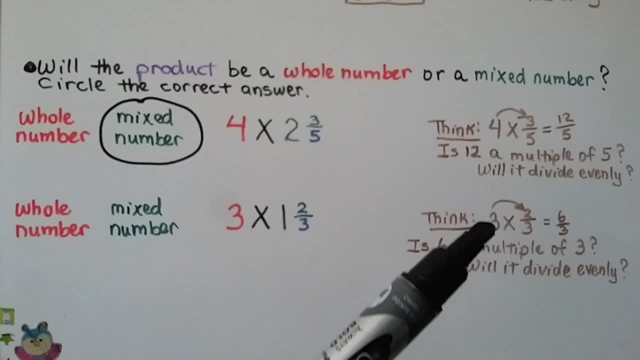 we're multiplying the 3 to the 2 thirds. we're going to multiply the 3 to the numerator 2 and get a 6 thirds. is 6 a multiple of 3? yes, it is. will it divide evenly? yes, because this is a 3 in that. 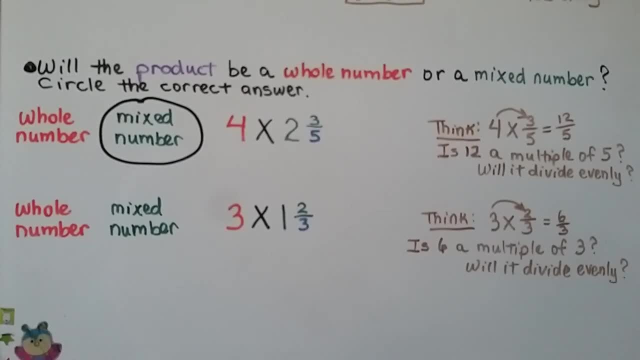 denominator's a 3. we know our answer is going to be a whole number and knowing how this works will help you check your answers quickly if you see that this is a 3 and that's a 3 and your product is a mixed number. you know you made a math. 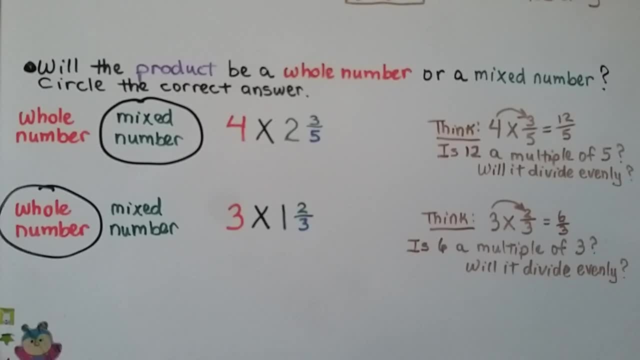 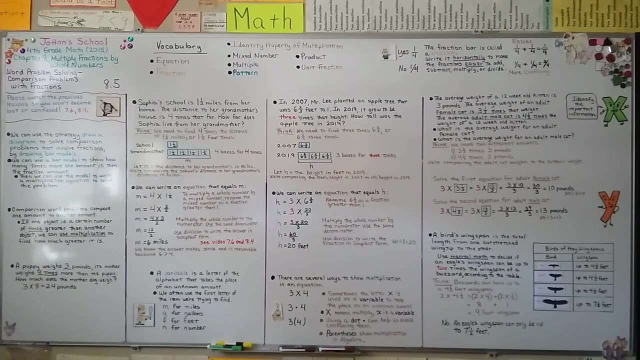 error and you need to go back and check your work. This is the last lesson for chapter 8, for multiplying fractions by whole numbers. We're going to move on to chapter 9. now We're going to talk about how fractions and decimals are related. 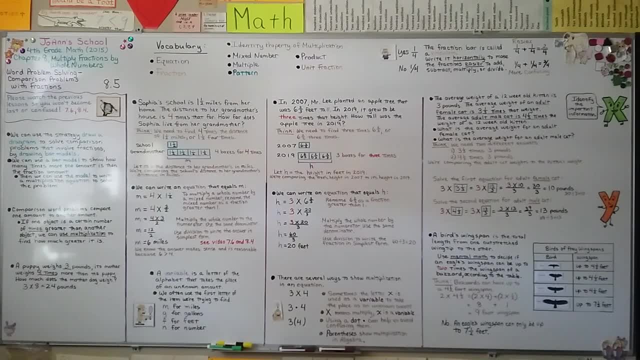 and I hope you have a really good day and I'll see you there. Bye you. 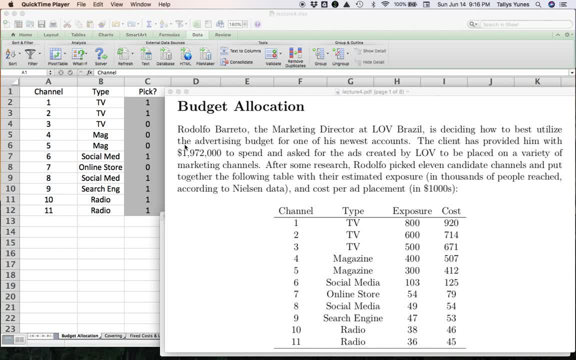 Hi again, everyone. So this is going to be our second video on the topic of integer programming. More specifically, we're still looking at binary variables. I'm going to assume that you have watched the video that comes right before this one, the first one on budget allocation, aka the 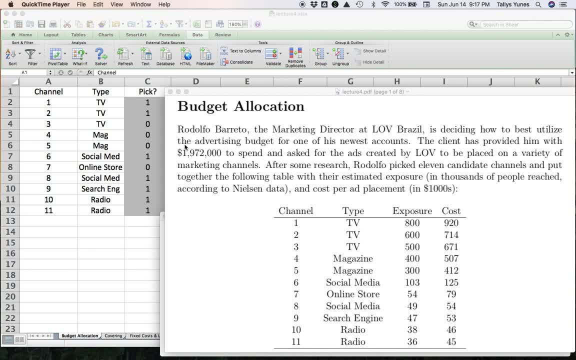 knapsack problem. If you haven't watched that video, please do that first. I'm going to put a link to it down in the description of this video below and as well as up here on the screen at the top right hand side corner. All right, so if you recall, we solved this budget allocation problem with the 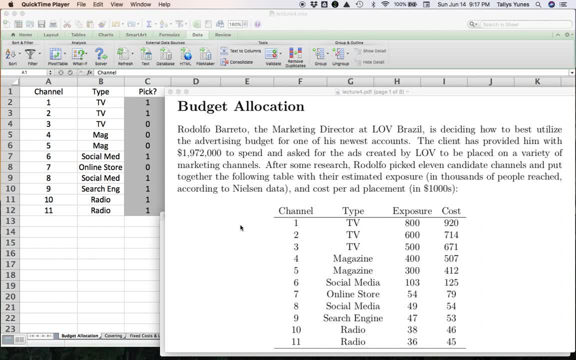 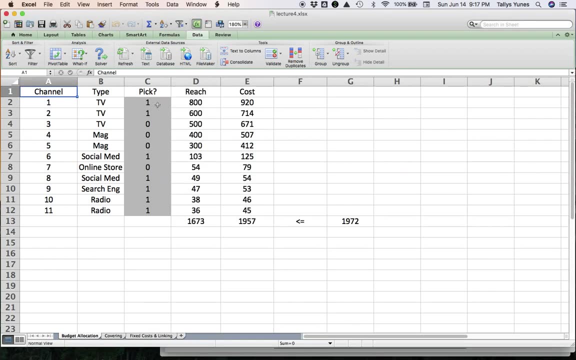 binary variables that decided whether or not to pick each of these advertising channels in order to maximize the overall reach- how many people see the ads for the product- and stay within the budget. And our answer was this right. So the ones indicate which channels. 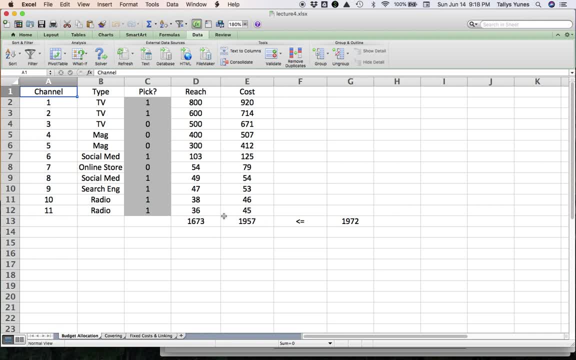 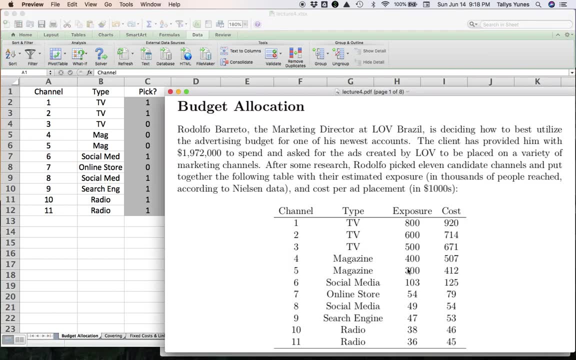 we picked how much money we spent out of our budget and how many people actually saw the ads. Now let's go ahead and do the following. With these yes-no decision variables, we can implement a few additional constraints to capture some situations. 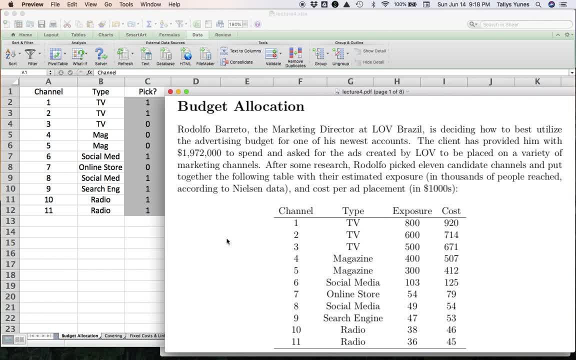 In this example we're going to look at the three main conditions that might be part of the real life problem we are interested in solving. These are called logical conditions. They are conditions that typically will involve some sort of If-then-else situation or some type of counting situation.